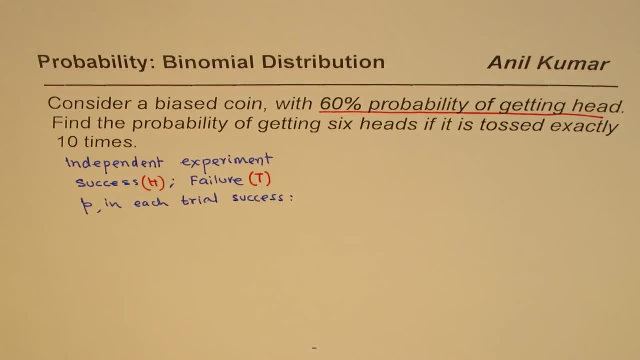 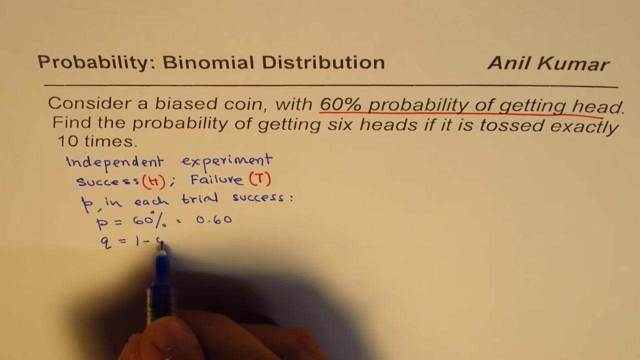 So for us, success is head. So this value of P is equal to 60% or 0.60.. Is it okay? So that is the probability of success. Now, what is the probability of failure, which is Q will be 1 minus 0.60.. So that is 0.40.. So that is the probability of failure. 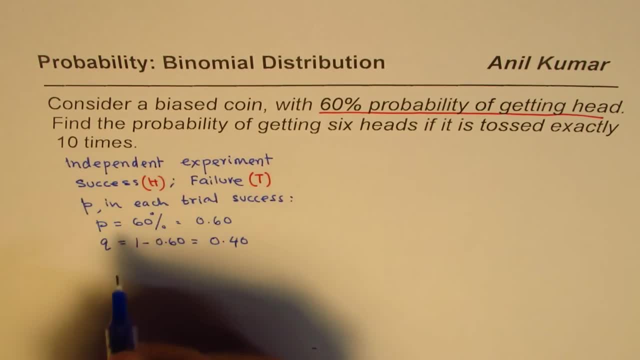 How many trials do we have? Exactly 10 times. So N, the number of trials is 10.. And what are we expecting? 6 heads. So we are expecting the random variable X will be number of heads in 10 trials. Is that okay? Number of heads in 10 trials? And we want this value of X equals to 6.. So small x is 6 for us, Correct? 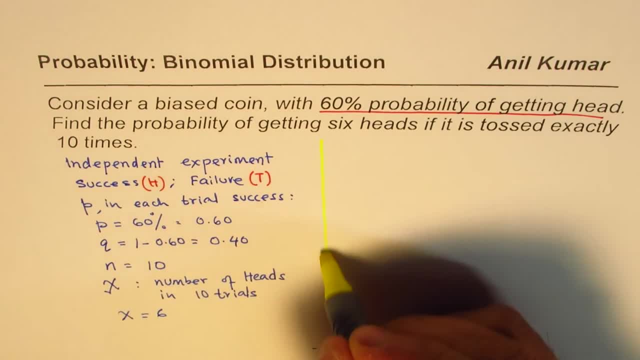 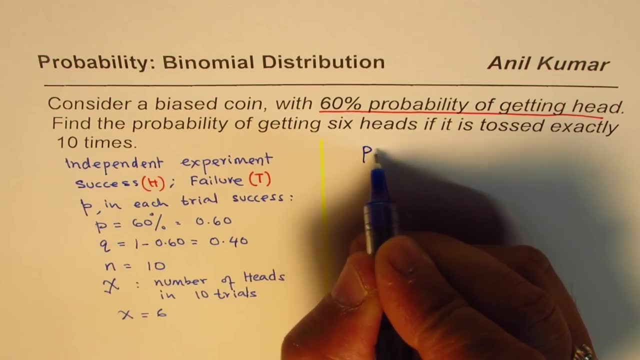 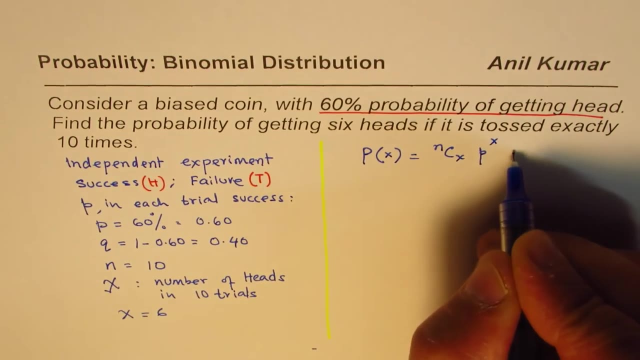 So all this is given to us. What do we need? What do we need to find Probability of getting 6 heads So we can use the formula. So, in general, the formula for binomial distribution is Ncx, lowercase p to the power of x, Q to the power of N minus x. Correct. 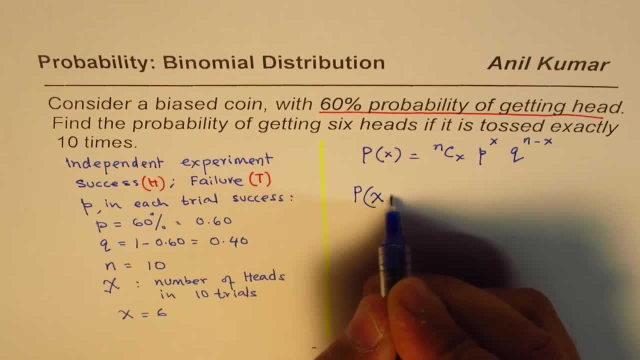 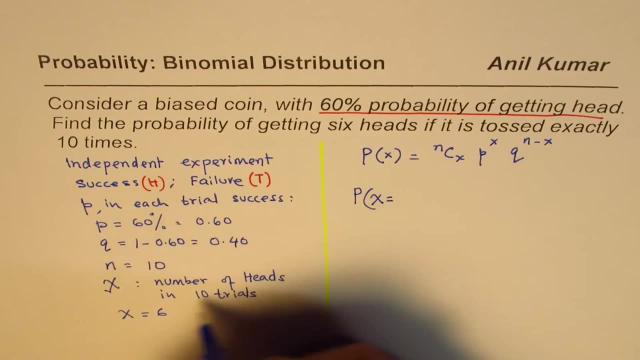 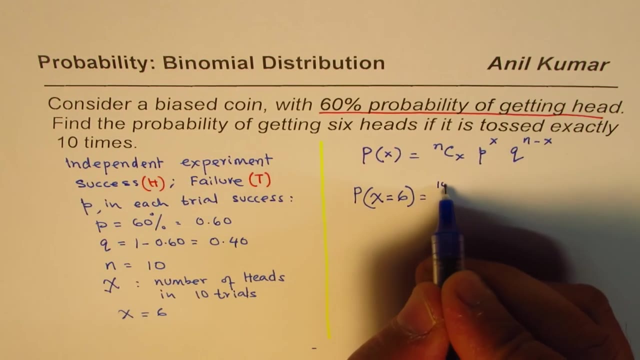 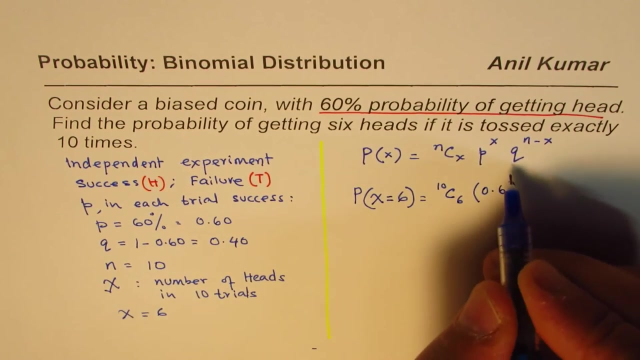 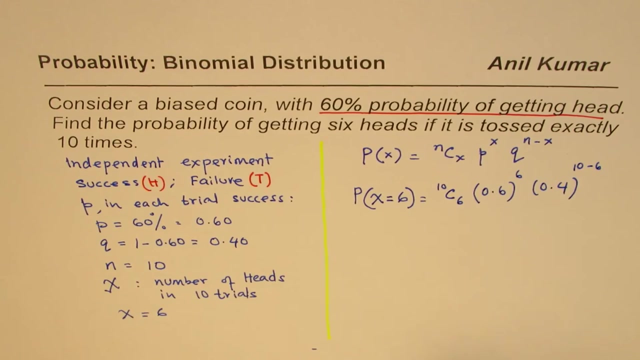 So we are looking for probability. when this parameter X is equal to, we say: find the probability of getting 6 heads Right. So the small x is 6.. So we can write X as 6.. N, we know, is 10.. All these values are known to us, So 10c6.. P is known to us. P is 60%, 0.6 to the power of 6.. Q is 0.4 now And it is 10 minus 6.. Is that okay? So that is how you can calculate. So it is 10c6,, 0.6 to the power of 6, and 0.4 to the power of 4.. 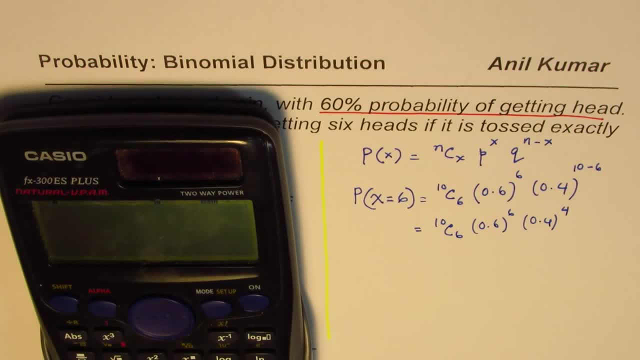 So we can use the calculator, Find the answer Right. So it is 10c6 times 0.6 to the power of 6 times 0.4 to the power of 4.. Right, And this is equal to. there is a narrow, Let's do it in steps, So 10.. Okay, let's clear this.